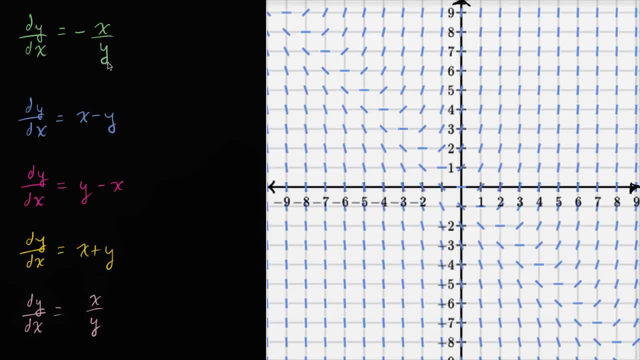 Start with a slope field and figure out which differential equation is the slope field describing the solutions for? And so I encourage you to look at each of these options and think about which of these differential equations is being described by this slope field. I encourage you to pause the video right now and try it on your own. 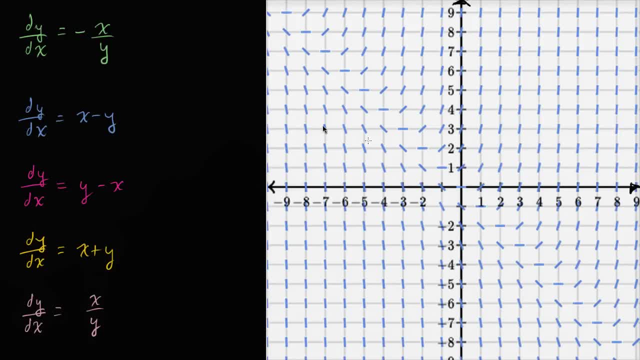 So I'm assuming you have had a go at it. So let's work through each of them, And the way I'm going to do it is: I'm just going to find some points that seem to be easy to do arithmetic with, and we'll see if the slope described by the differential equation at that point. 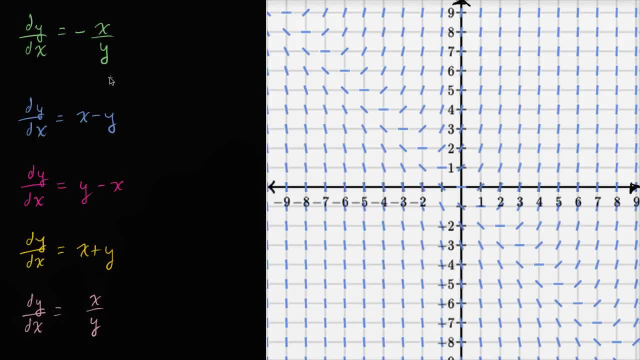 is consistent with the slope depicted in the slope field And I don't know. just for simplicity, maybe I'll do x equals 1, y equals 1 for all of these. So I'm going to see what. so when x equals 1 and y is equal to 1.. 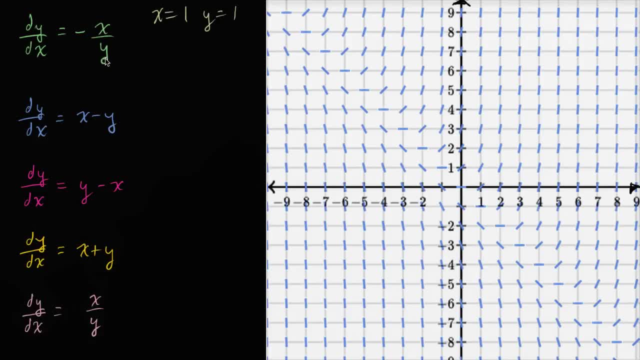 So this first differential equation right over here: if x is 1 and y is 1, then dy dx would be negative, 1 over 1 or negative 1.. dy dx would be negative 1.. Now is that depicted here When x is equal to 1 and y is equal to 1,? 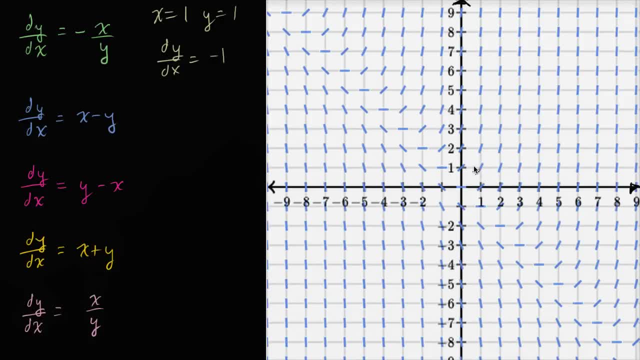 our slope isn't negative: 1,. our slope here looks positive, So we can rule this one out. Now let's try the next one. So if x is equal to 1 and y is equal to 1,, well then dy dx would be equal to 1 minus 1 or 0.. 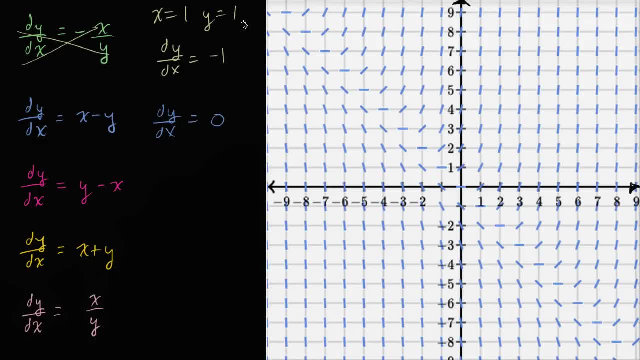 And once again I just picked x equals 1 and y equals 1 for convenience. I could have picked any other. I could have picked negative 5 and negative 7.. This just makes the arithmetic a little easier, Once again when you look at that point that we've already looked at. 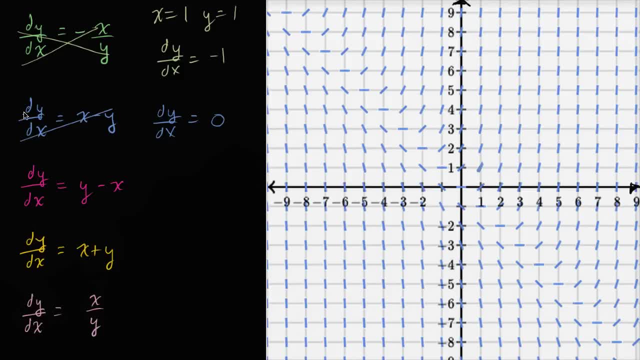 our slope is clearly not 0. We have a positive slope here, So we could rule that out Once again for this magenta differential equation: if x and y are both equal to 1, then 1 minus 1 is once again going to be equal to 0. 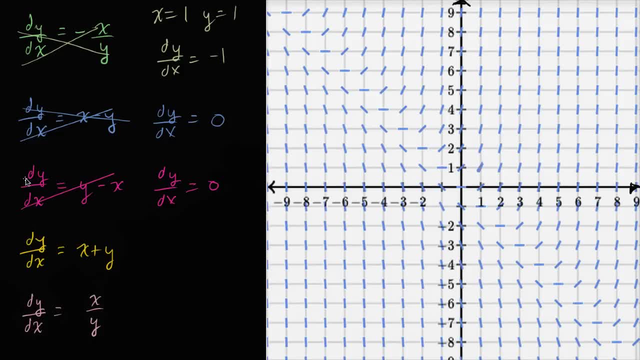 And we've already seen the slope is not 0 here, So rule that one out. And now here we have x plus y. So when x is 1, y is 1, the derivative of y with respect to x is going to be 1 plus 1.. 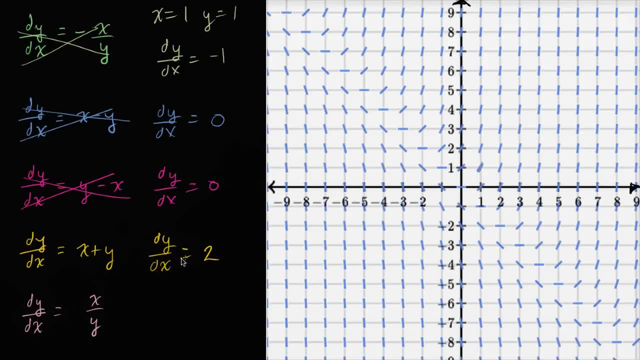 Which is equal to 2.. Now this looks interesting. It looks like this slope right over here could be 2.. This looks like 1, this looks like 2.. I want to validate some other points, but this looks like a really really good candidate. 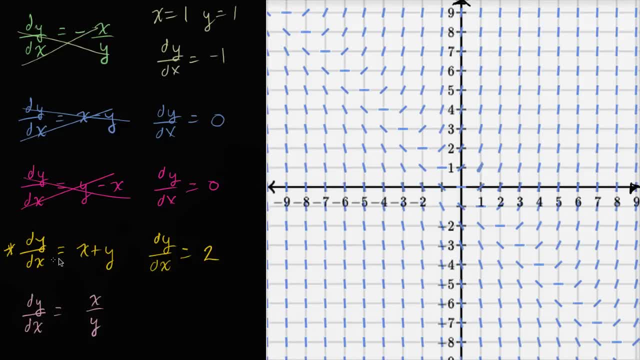 And you could also see what's happening here. When dy dx is equal to x plus y, you would expect that as x increases for a given y, your slope would increase, And as y increases for a given x, your slope increases, And we see that. 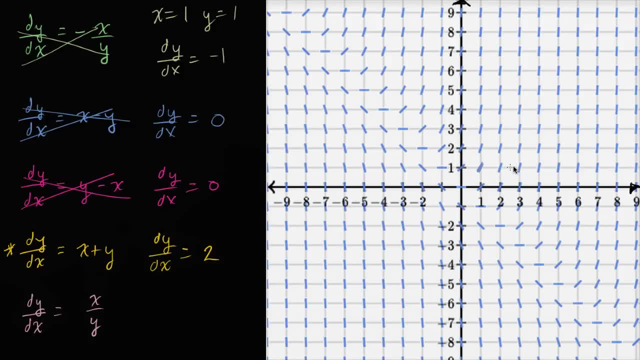 If we were to just follow, if we were to hold y constant at 1, but increase x along this line, we see that the slope is increasing, It's getting steeper. And if we were to keep x constant and increase y across this line? 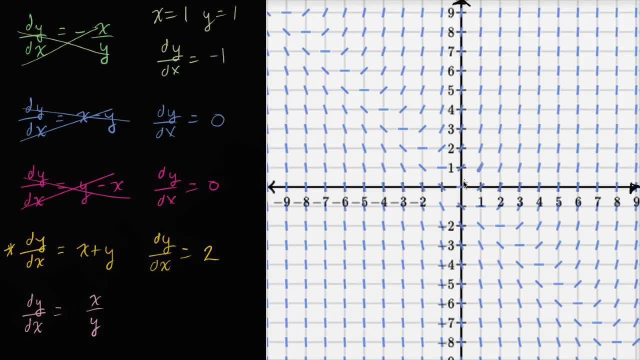 we see that the slope increases And in general, we see that the slope increases as we go to the top right And we see that it decreases as we go to the bottom left, And both x and y become much, much more negative. 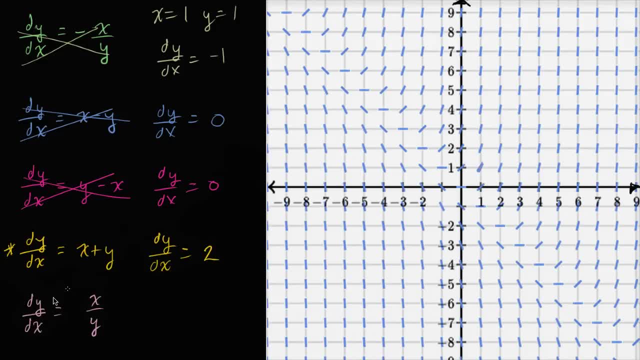 So I'm feeling pretty good about this, especially if we can knock this one out here, if we can knock that one out. So dy dx is equal to x over y. Well then, when x equals 1,, y equals 1,. 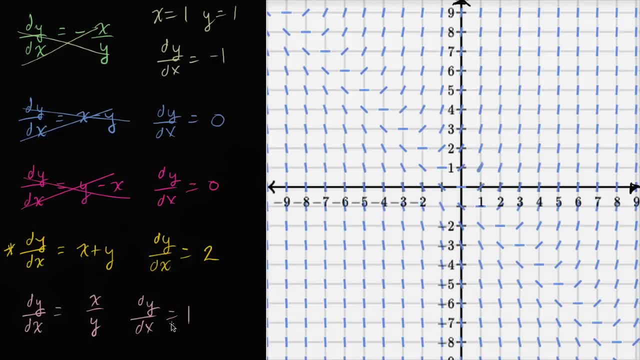 dy dx would be equal to 1. And this slope looks larger than 1.. It looks like 2, but since we're really just eyeballing it, let's see if we can find something more clearly where this more clearly falls apart. 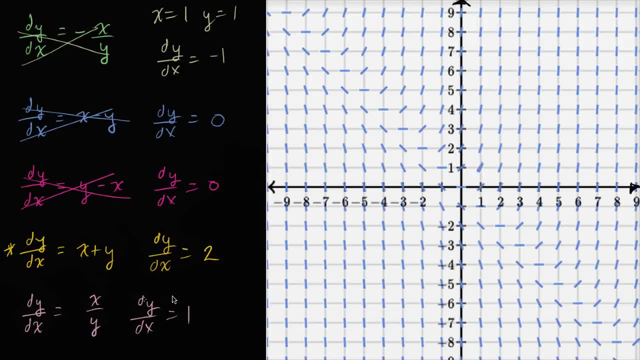 So let's look at the situation when. let's look at the situation when they both equal negative 1.. So x equals negative 1, and y is equal to negative 1.. Well, in that case, dy dx should still be equal to 1,. 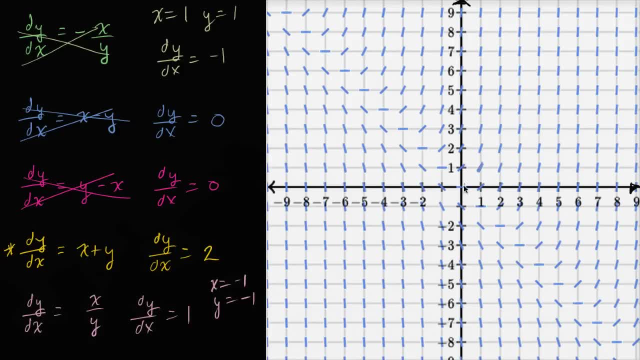 because you have negative 1 over 1.. Do we see that over here? So when x is equal to negative 1, y is equal to negative 1, our derivative here looks negative. It looks like negative 2, which is consistent with this yellow differential equation. 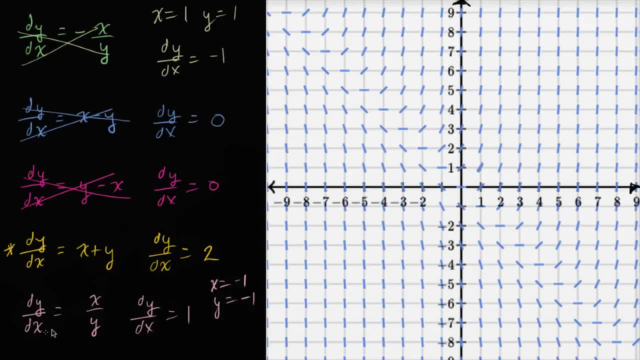 And the slope here is definitely not a positive 1.. So we could rule this one out as well, And so we should feel pretty confident that this is the differential equation being described, And now that we've done it, we can actually think about. 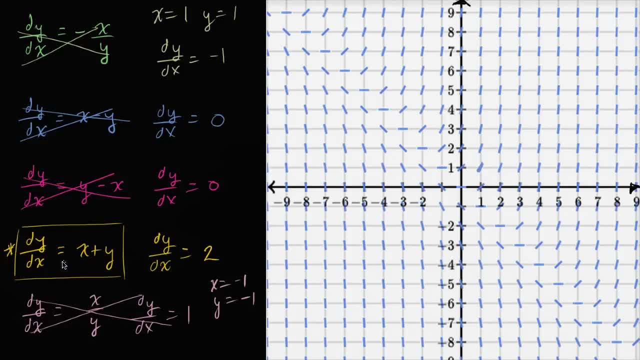 well, okay, what are the solutions for this differential equation going to look like? Well, it depends where they start, If you have, or what points they contain. If you have a solution that contains that point, it looks like it might go. 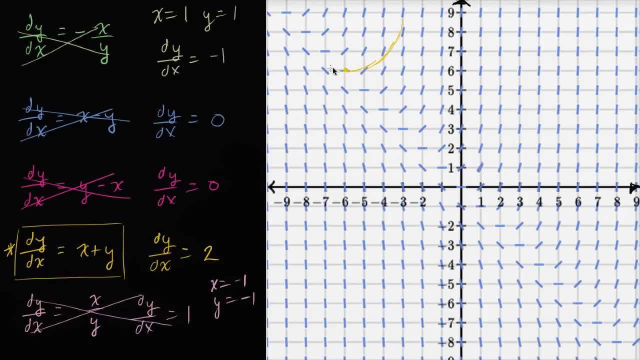 looks like it might do something. looks like it might do something like something like this: If you had a solution that contained- I don't know if you had a solution that contained- this point- it might do something. it might do something like that. 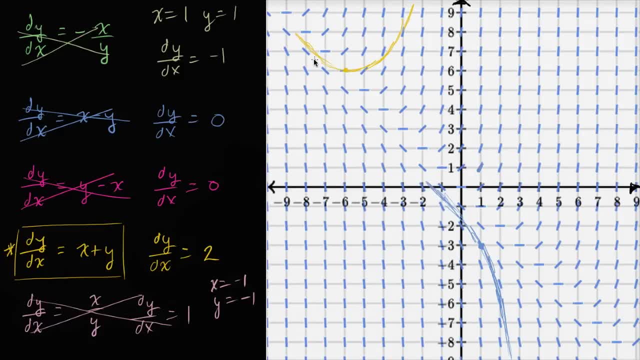 And of course it keeps going. It looks like it would asymptote towards y is equal to negative x. this downward sloping, this, essentially, is the line y is equal to negative x. Actually, no, that's not line equals y equals negative x. 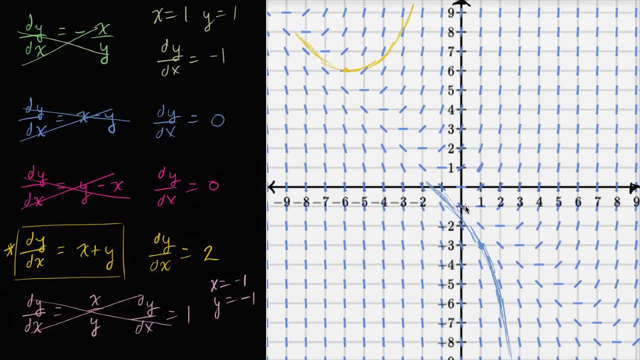 This is the line. y is equal to negative x minus one. So that's this line right over here And it looks like if you had, if you had your in a solution, if you had a, if the solution contained, say this point right over here. 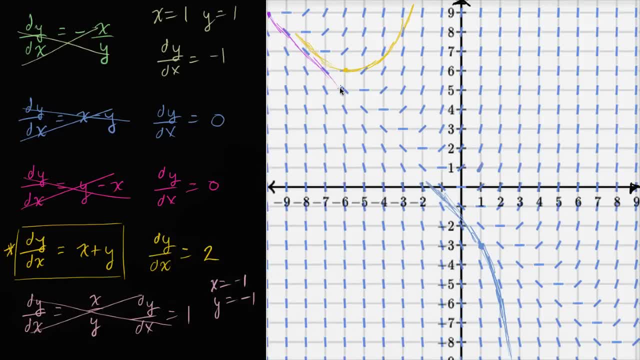 you would actually. that would actually be a solution to the differential equation. y is equal to. y is equal to negative x. whoops, y is equal to negative x minus one, And you can verify that If y is equal to negative x minus one.